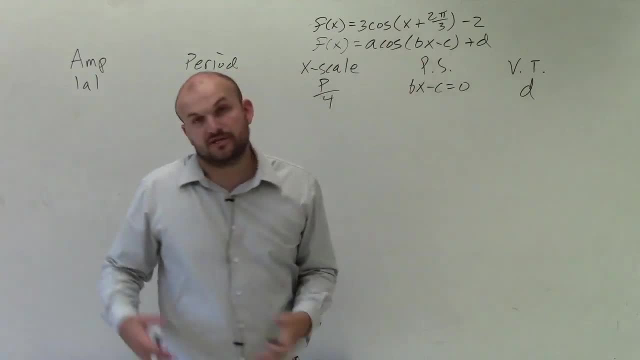 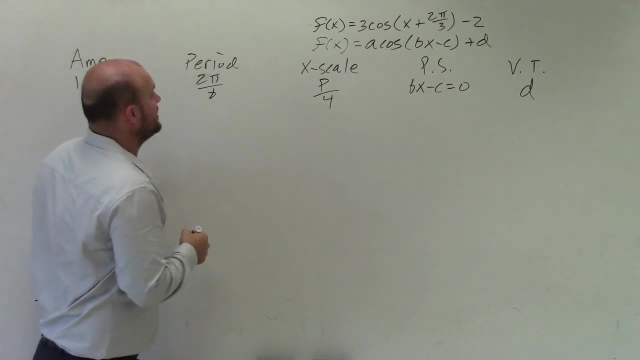 to do is look at our values for a, b, c and d in our equation and just plug them in, So So absolute value of a s value 3 is equal to 3.. For a period you have 2 pi divided by b. 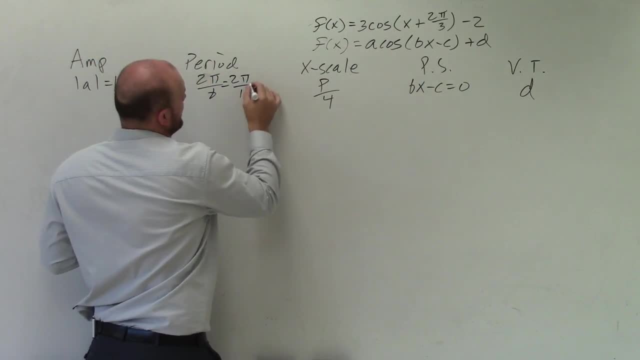 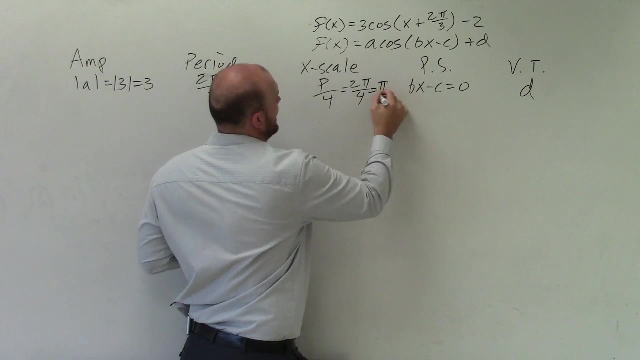 Well, b in this case is 1.. So it's just 2 pi divided by 1, which is just 2 pi. Our period is just going to be 2 pi over 4, which equals pi halves. Our phase shift is going to be set whatever's. 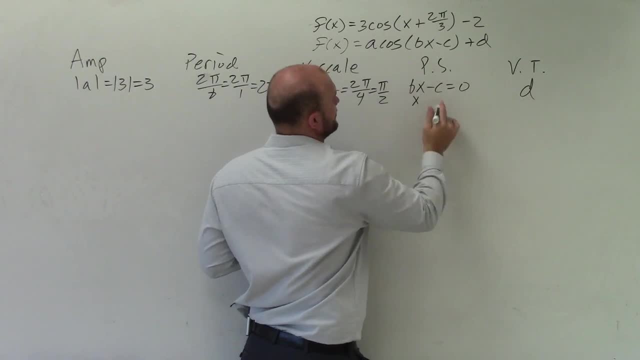 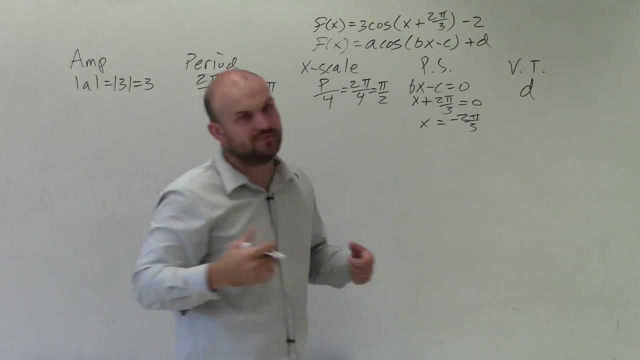 inside of our parentheses. So x plus 2 pi over 3 equals 0.. x equals negative 2 pi over 3.. You have to subtract 2 pi over 3 on both sides And then d is going to equal negative 2.. 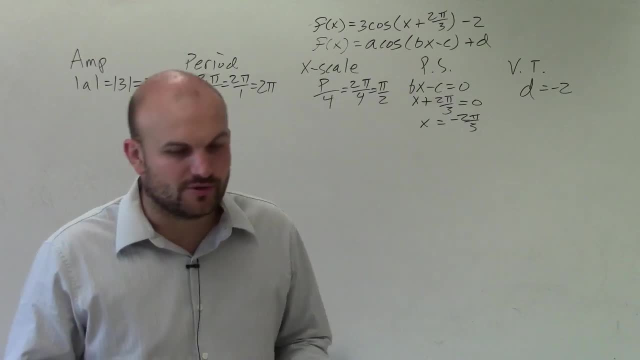 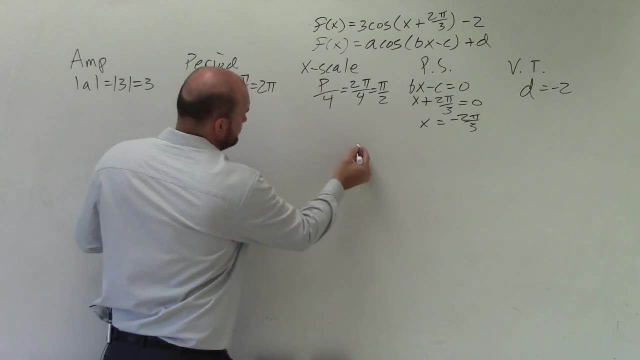 That means I'm going to shift my graph down two units. So now that we have an amplitude, we kind of need to understand what exactly is amplitude going to be doing to our graph. Let's start at 0 here And now. when I'm graphing a trigonometric function. 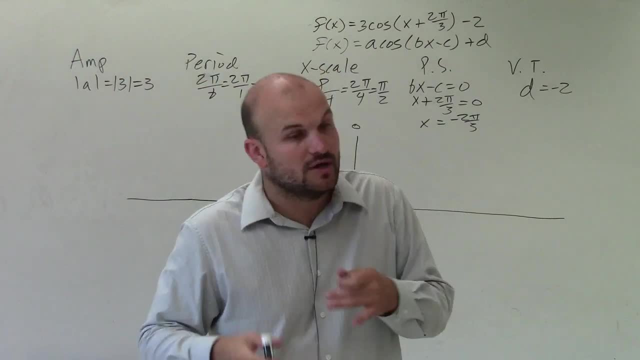 a lot of times we start at our initial period at 0.. And we say 0, and you can do two periods to the right, two periods to the left, Two periods to the left, a period to the right, a period to the left. 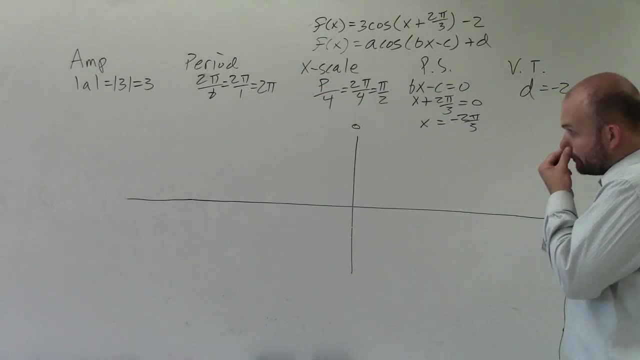 Doesn't really matter In this case, I'm going to do a period to the left and a period to the right. Now, this is going to go ahead and get fun Because, first of all, we know our amplitude. Remember, amplitude is the half distance from the maximum. 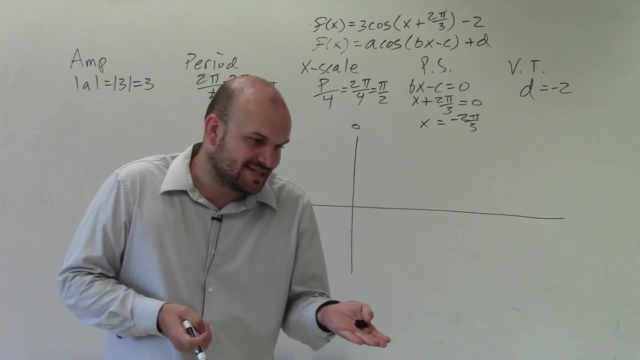 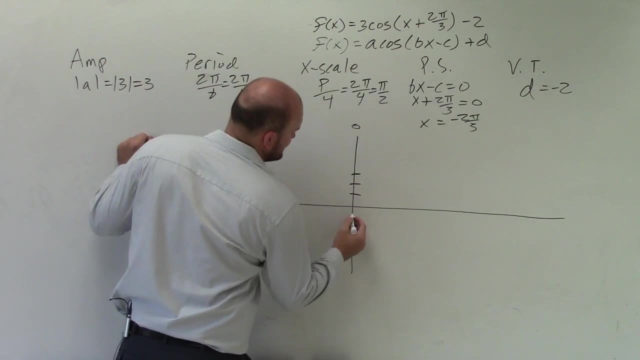 to the minimum Pretty much the distance from wherever your graph crosses the x-axis to its maximum or its minimum. So since that is 3,, I'm going to go up 3,, 1,, 2, 3, and down 3,. 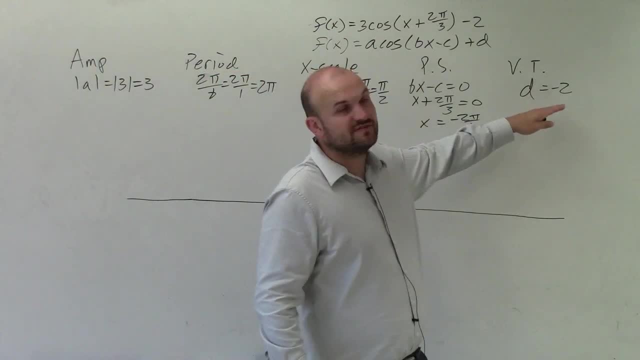 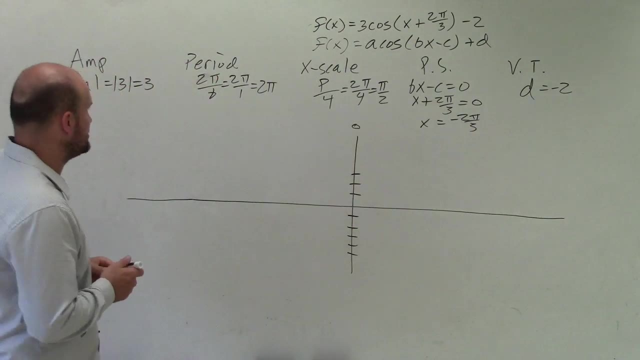 1,, 2,, 3.. However, I do also notice that I'm going to be shifting the graph down two units, So down 2.. So I'm going to have to go 1,, 2,, 3. And I'll show you guys that in just a minute. 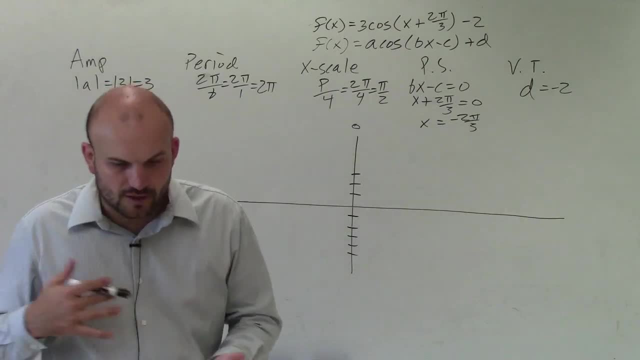 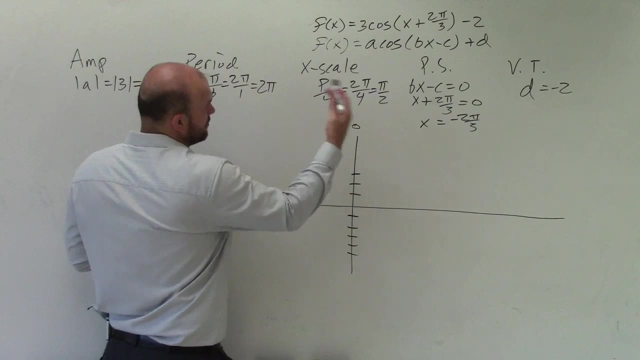 The main important thing, I think is the hardest thing to do right now- is to be able to identify the x-scale. All right, So rather than starting at 0, which the parent graph is at, we're going to start at negative 2 pi. 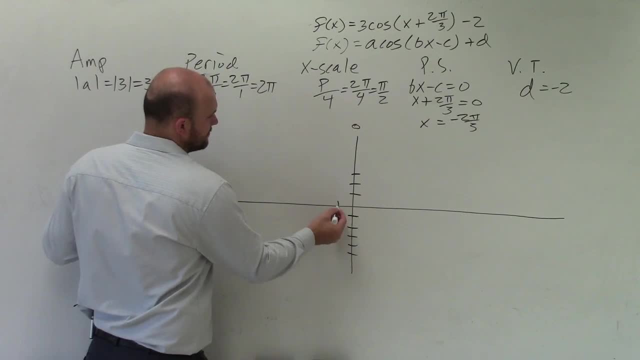 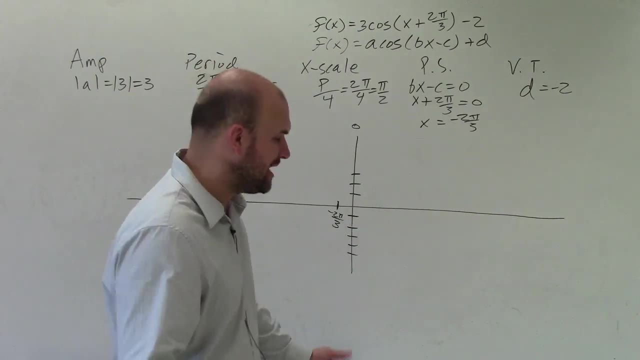 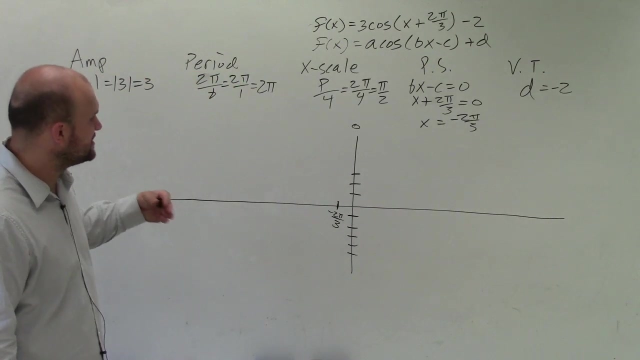 over 3.. So let's just say negative 2 pi, Rosa. would you come To the front office please, Rosa? OK, So we have negative 2 pi over 3.. Now the main important thing for us to understand: 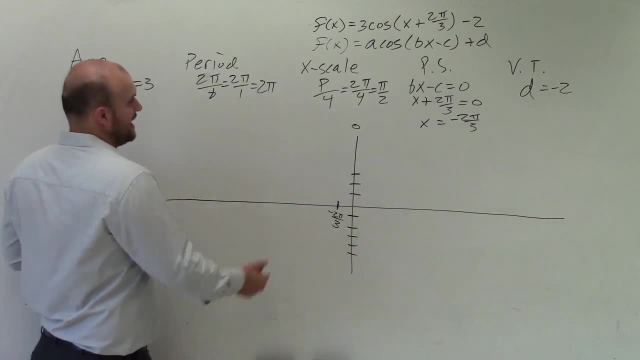 is: remember we're going to be doing our x-scale And we need to go to our x-scale to the left and to the right in this case. Or you can do 2 to the right, But remember there's four x-scales in each period. 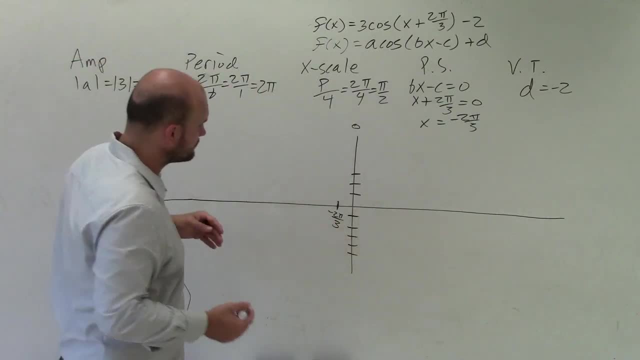 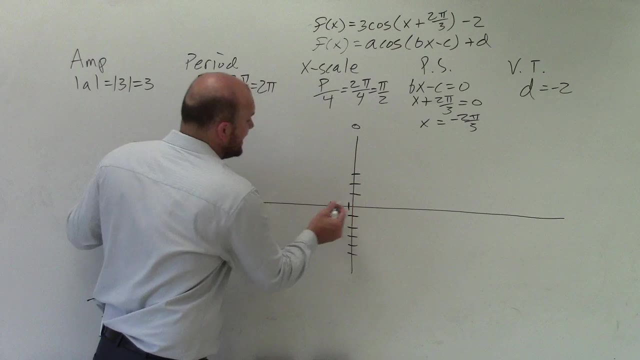 So to find my next scale, let's make it right there, All right. To find my next point, I'm going to have to add: that's going to be over pi halves to the right. So what I need to do is let's see a little work here. 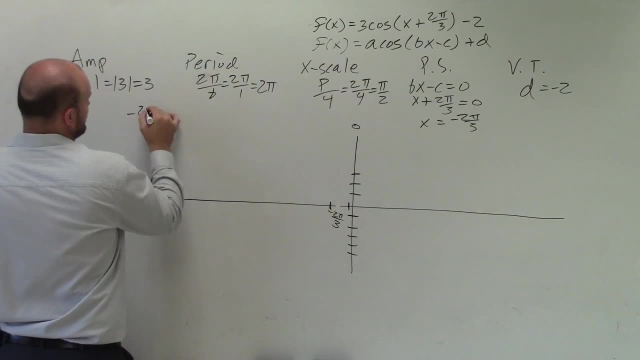 Let's do it over here, So I can simply just take negative 2 pi over 3 plus pi halves. Now obviously I've got to get them to be common denominators, to add these up together. So I multiply by 2 over 2,, 3 over 3, and what I get is negative 4 pi. 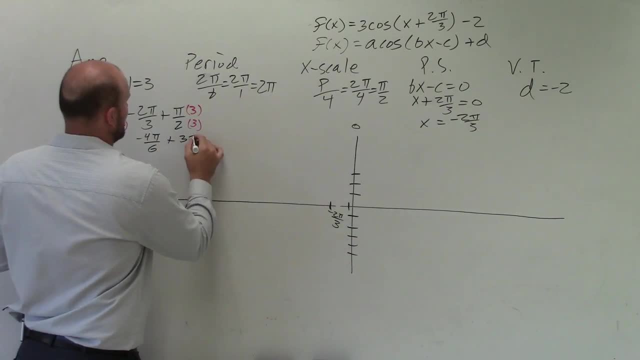 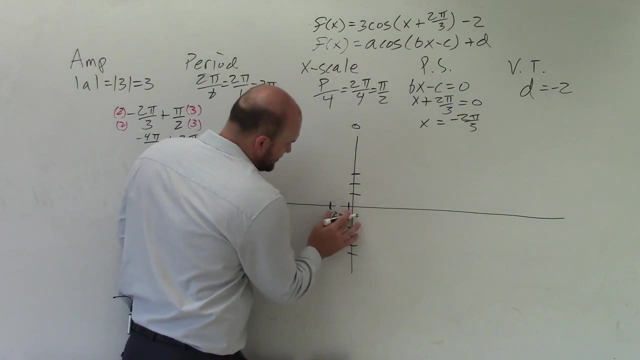 over 3.. All right, Negative 4 pi over 6 plus 3 pi over 6,, which equals negative pi over 6.. So therefore, this next value is negative pi over 6.. All right, Then I need to add another scale, another scale. 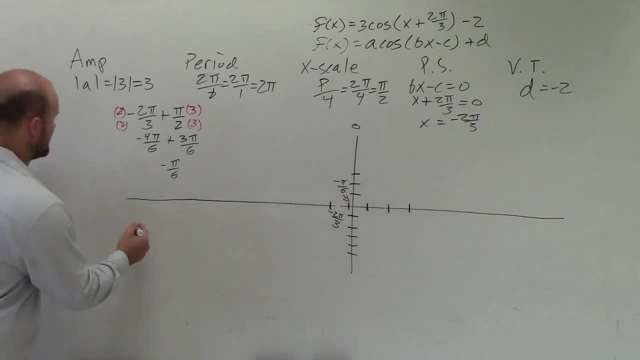 and another scale. So I'm going to keep on adding pi halves. So now I just take negative pi halves plus negative pi over 6. Plus pi halves Again, I need to get common denominators, So I'll multiply by 3 over 3.. 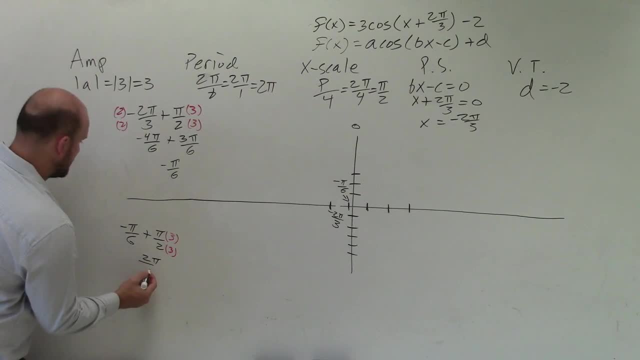 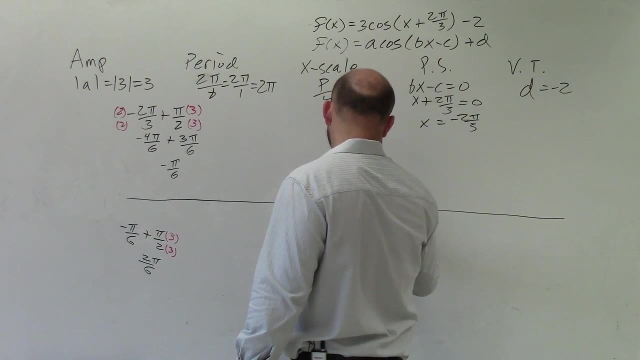 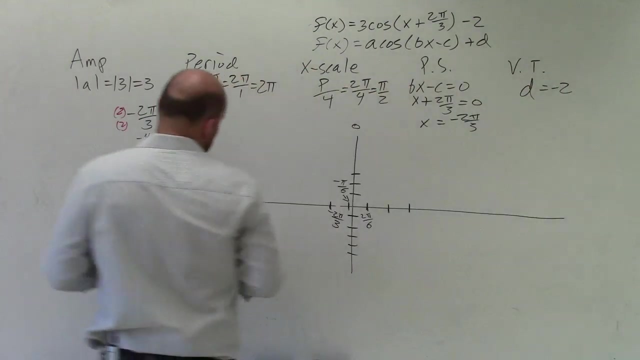 In this case, I have 2 pi over 6.. Now what I like to do is, rather than simplify each one of these, I like to kind of keep them in the same order So I can say: well, what am I adding from negative pi? 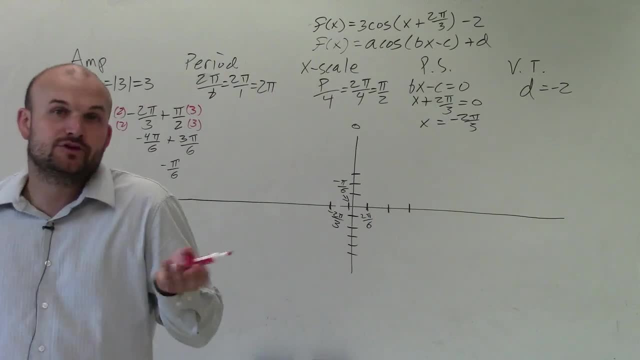 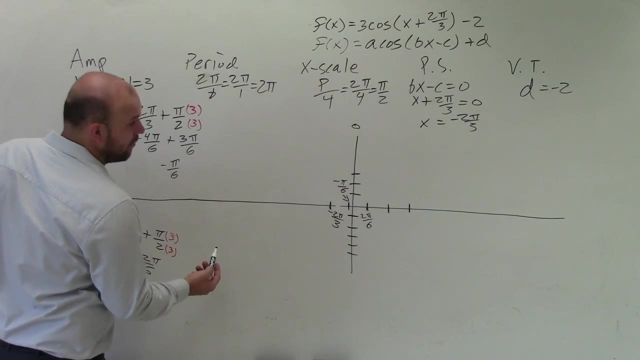 over 6 to 2 pi over 6? You're pretty much adding. You're adding 3 units up top And let's just go and see Is that going to make sense as well going backwards, Because simply that would be negative 4.. 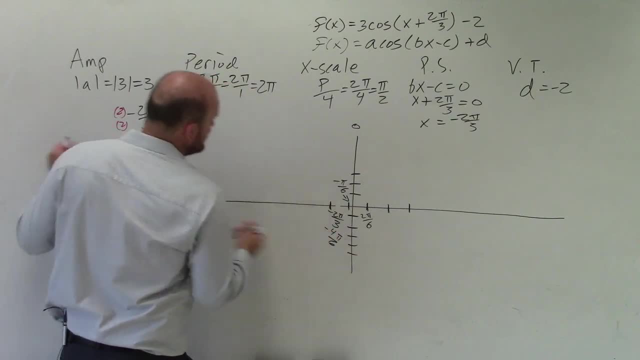 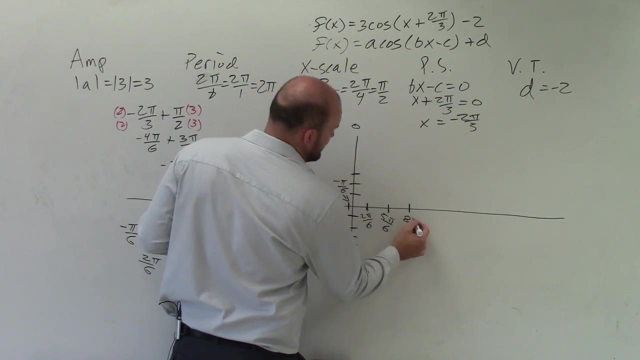 Yeah, So really this is like negative 4 pi over 6.. Now you can keep on doing the algebra if you want to, But I've figured out the pattern of adding. it is really just like 5 pi over 6 and 8 pi over 6.. 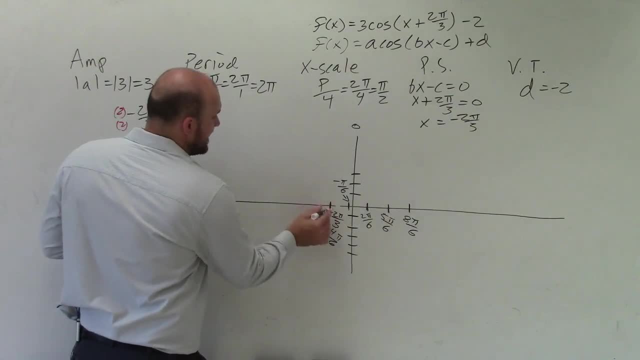 Now, again, I will go back and simplify them, But again, remember, here's our starting point, right? So I'm going to do a period to the right as well as a period to the left. So I'll do 1,, 2,, 3,, 4.. 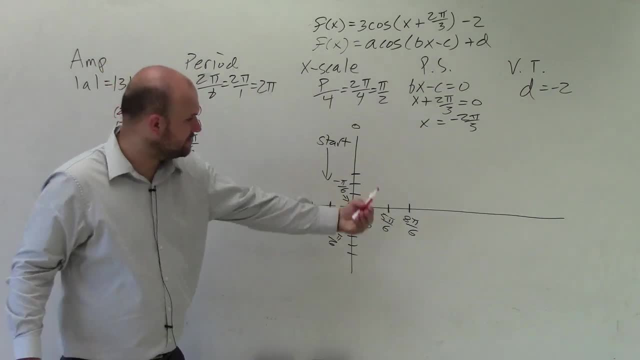 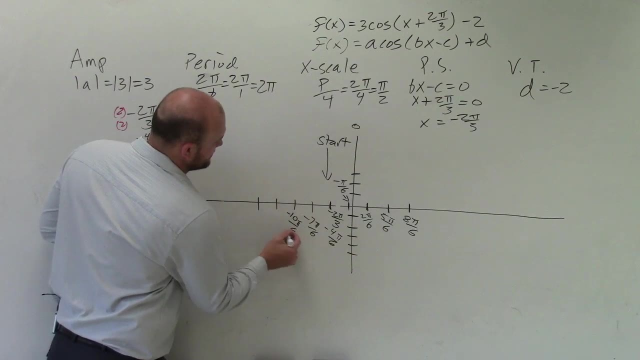 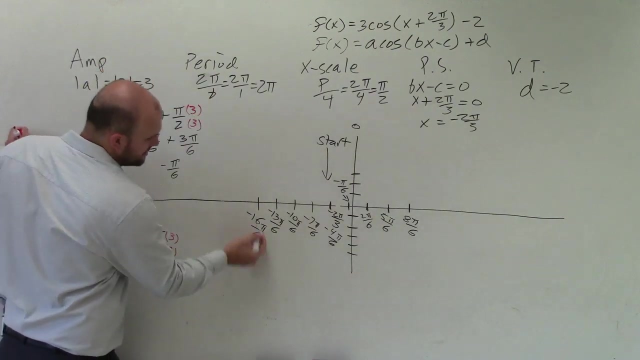 So now, rather than adding, I'm now going to subtract. So negative 7 pi over 6, negative 10 pi over 6, negative 13 pi over 6, and negative 16 pi over 6.. And then, for each one of these, I'm simply: 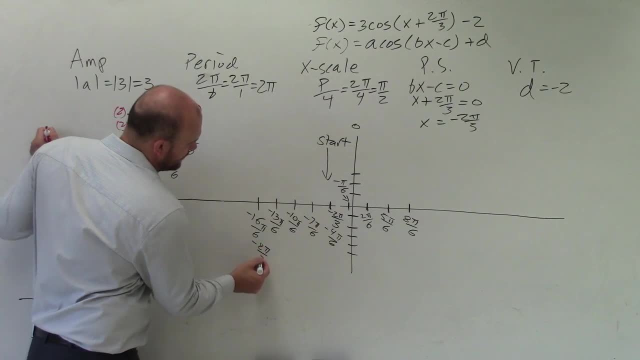 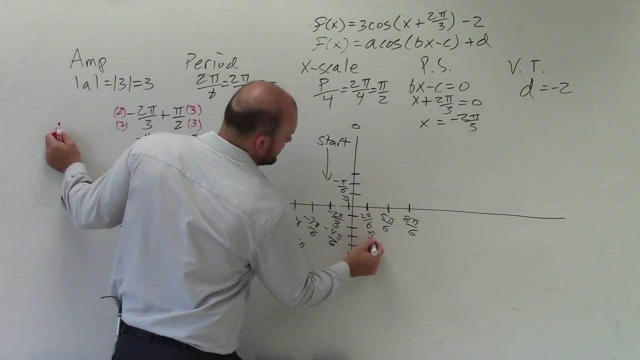 just going to go ahead and reduce. That's really negative: 8 pi over 3.. That's negative: 5 pi over 3.. That's negative: 2 pi over 3,, which you're already did. That is really pi over 3.. 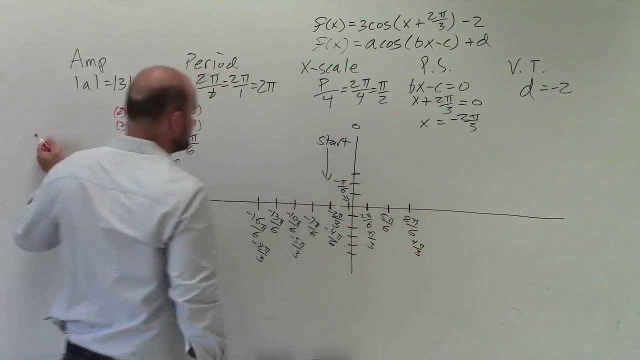 And that is really 4 pi over 3.. So I know that's kind of like. you're like whoa, way too much information, right? So let's get on the ones that we. oh shoot, I like that one. 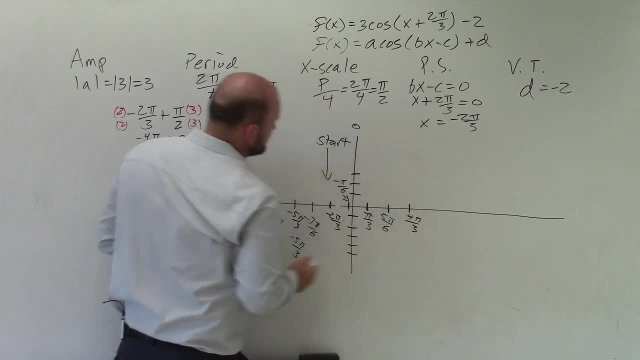 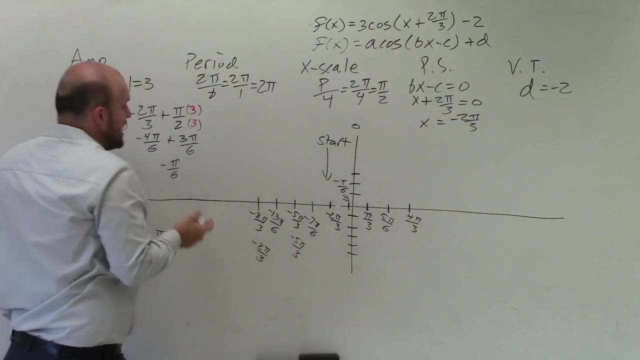 And 4 pi over 3.. OK, so now I got my scale And remember. here's where we start right Now. remember, I said that this graph is going to shift down two units Now first of all. so if we're going, 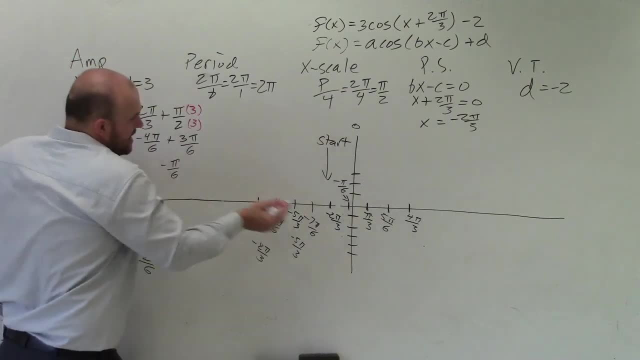 to be shifting down two units. what I'm going to simply do is take my x-axis and shift it down two units, And I'm going to represent the x-axis with a dashed line. Now, since I have this as a dashed line, 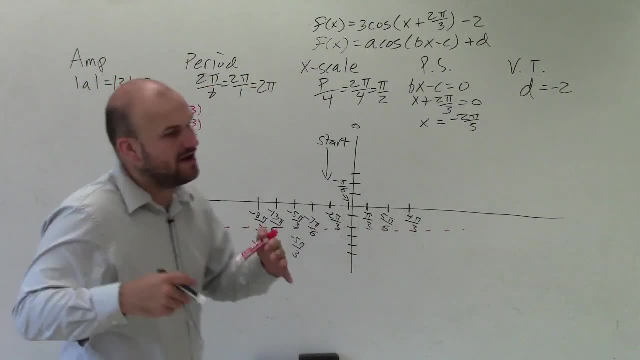 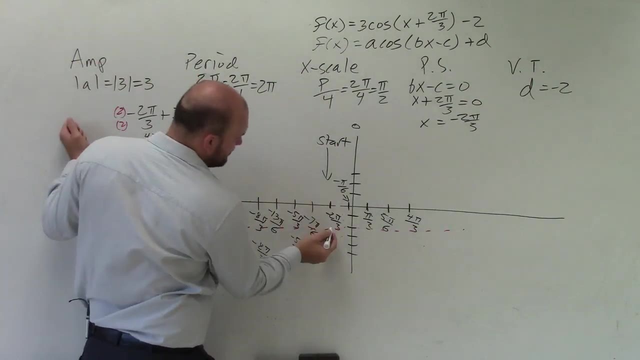 we also got to remember how high are we going up. Remember, the cosine graph, at its initial period, starts at its maximum right. Well, the maximum in this case has an amplitude of 3.. So from my starting point right here. 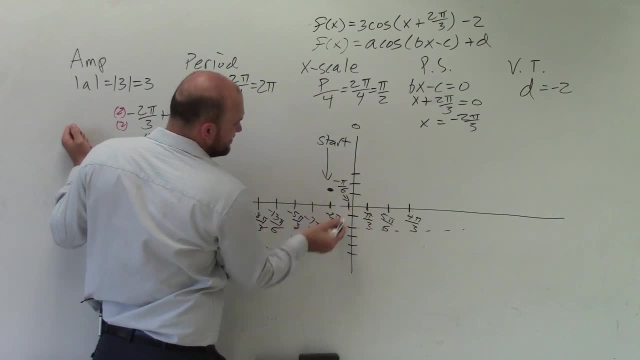 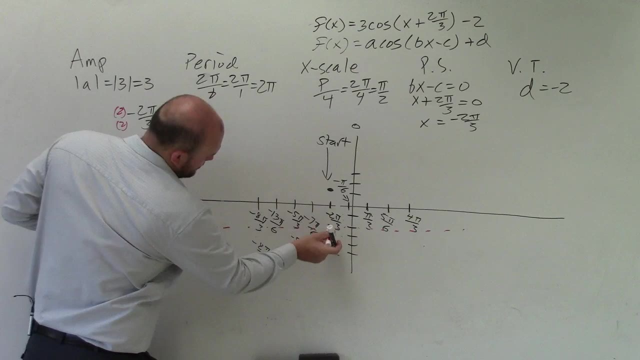 I'm going to go up three units- 1,, 2, 3, because that's going to be the highest. Then I need to go down three units. from this point, These are like swayed in the wrong direction. Then I need to. so I start here.